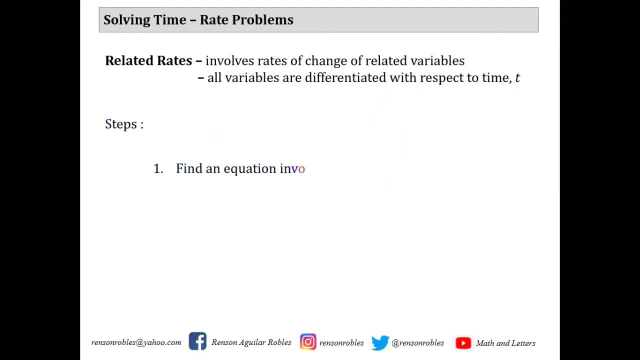 simple steps that you might want to follow. Step number one is to find an equation involving the variables, which is true for any time t. Number two is to differentiate the equation in obtained in step one with respect to the time t. And number three determine the unknown time rate. 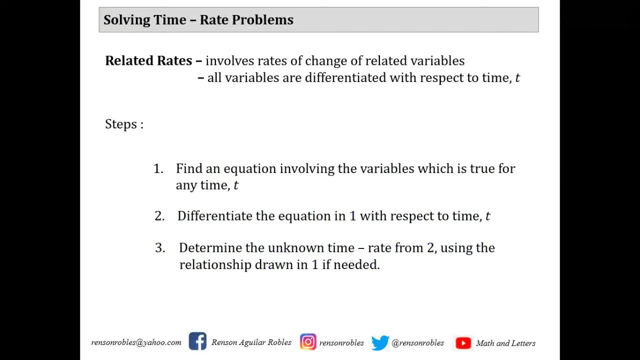 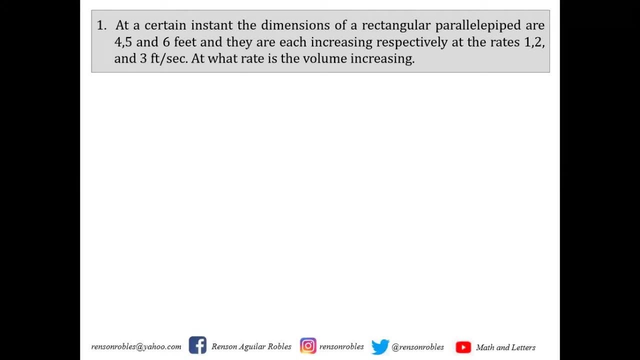 variable from step number two, using the relationship drawn in step number one if needed. And let me just give you an illustration. I have here a problem which involves rectangular parallelepiped. At a certain instant that the dimensions of a rectangular parallelepiped are four, five and six feet, and they are each increasing respectively at the rates of one. 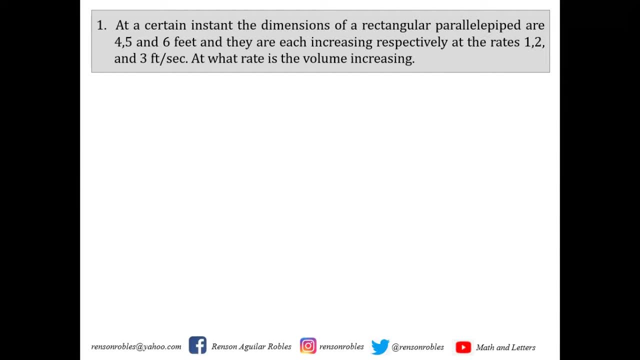 two and three feet per second. At what rate is the volume increasing? Just to illustrate the rectangular parallelepiped, we shall let x to be the width of the rectangular parallelepiped. The pipe width corresponds to its rate of change in width, which is denoted by d, x, dt. 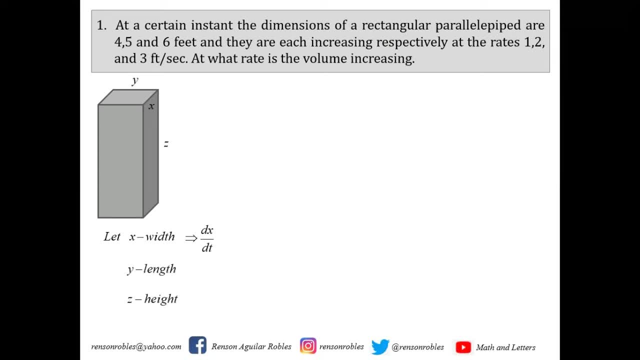 and y to the length and z to be the height, with corresponding dy, dt as the rate of change in length with respect to the time t, and dzdt is the rate of change in altitude or height with respect to the time t, and we shall recall that the volume of a rectangular parallelepiped. 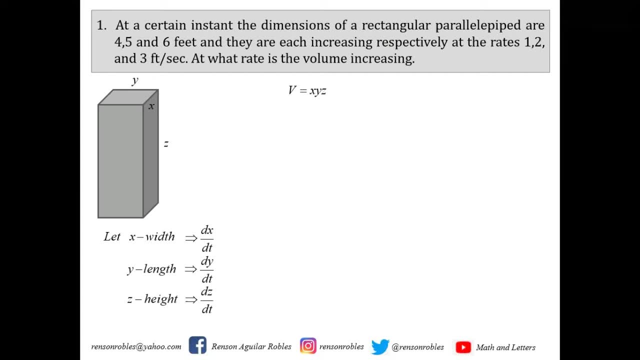 is length times width, times height, which is equal to x y z. So we shall differentiate this equation and this will serve as our working equation with respect to the time t. so we have db. dt equals derivative of x y z in terms of uh, derivative of x in terms of t. so 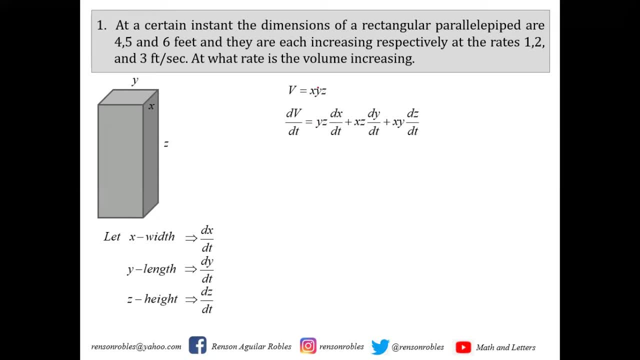 we have y, z, dx, dt plus uh. we shall now differentiate y in terms of t, so that's x, z, dy, dt plus uh. we shall do it in z. so we differentiate z with respect to the time t, just copy x, y, since this is constant, and differentiating z with respect to the time t is dz, dt. so at a certain instant, 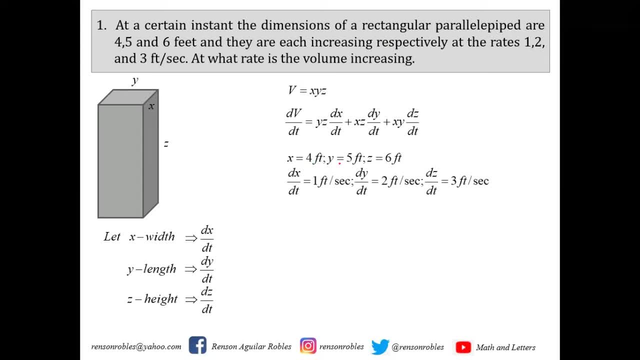 that the width is equal to four feet, that the length is five feet and that the altitude is six feet. the rate of change of width with respect to the time t is one foot per second, dy dt is two feet per second and dc dt equals three feet per second by direct substitution to this. 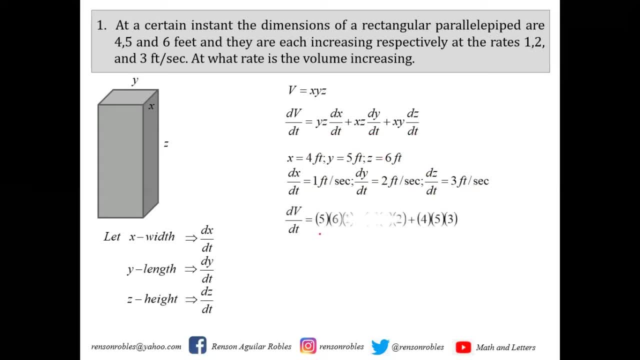 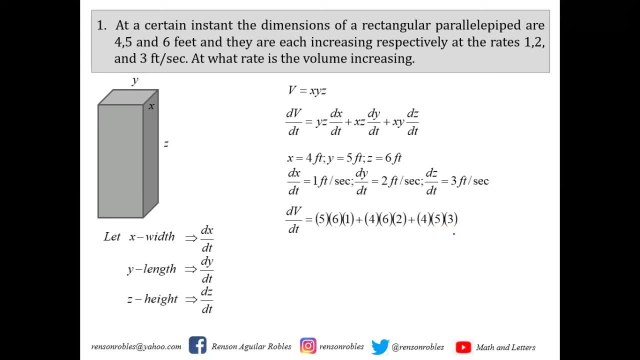 times five, which is your y times three, which is your dz dt, and solving this uh equation, db dt is equal to 138 cubic feet per second. so therefore, in conclusion, in a certain instant, that the dimension of rectangular parallely piped is four, five and six feet respectively, and 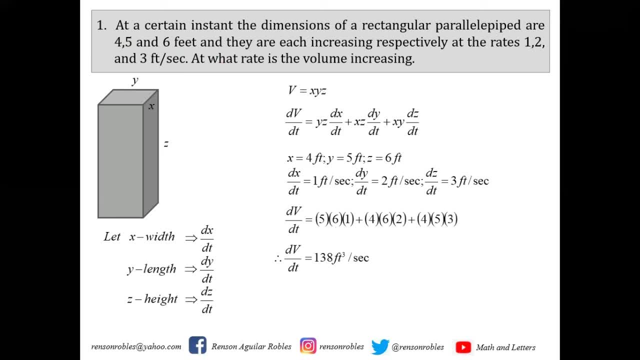 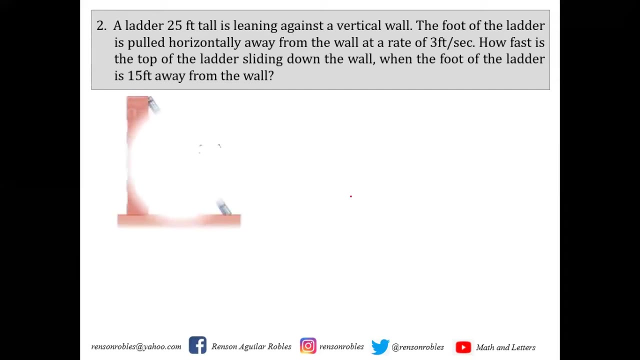 each uh dimension is increasing at a rate of one, two and three feet per second. then the volume is increasing at a rate of 138 cubic feet per second. another example: a ladder 25 feet tall is leaning against a vertical wall. the foot of the ladder is pulled. 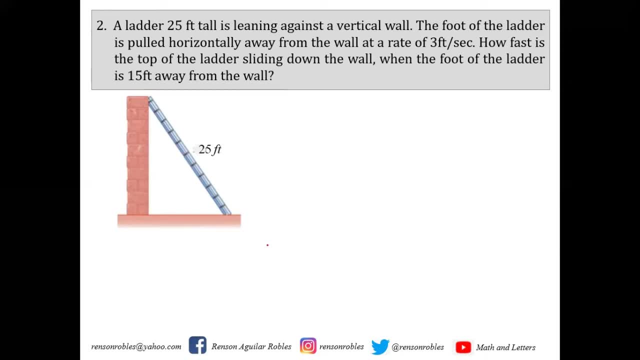 horizontally away from the wall at a rate of three feet per second, how fast is the top of the ladder sliding down the wall when the foot of the ladder is 15 feet away from the wall? so at a certain instance when you pull, when you pull the foot of the ladder away from the wall, so there will 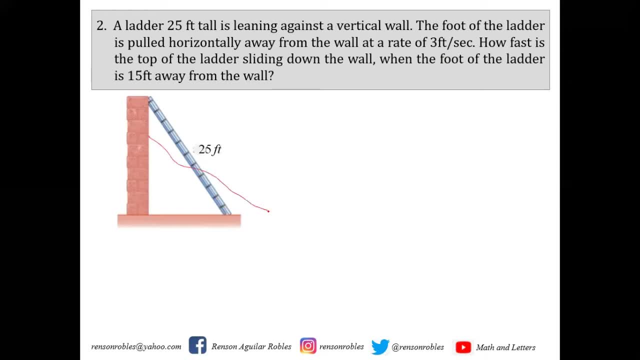 come to a point that the ladder will look like this: okay. so, or when you pull it, uh, towards the wall, it there will come to a point that the ladder will look like this: okay, and with that we shall let x to be the distance of the foot of the ladder. 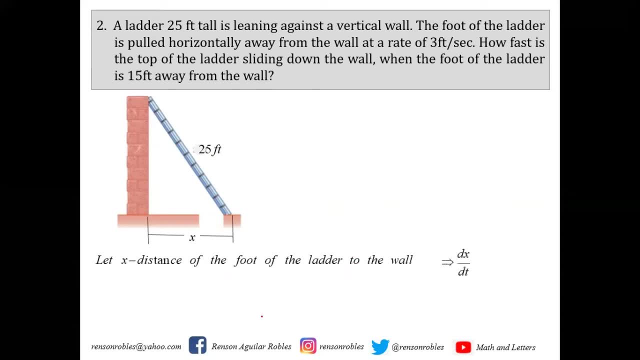 to the wall, and we shall let y to be the distance of the top of the ladder to the ground, with its corresponding rate of change. we shall let dx dp to be the rate of change in x with respect to the t and dy, dt is the rate of how fast the top of the ladder is sliding up and down the wall and then. 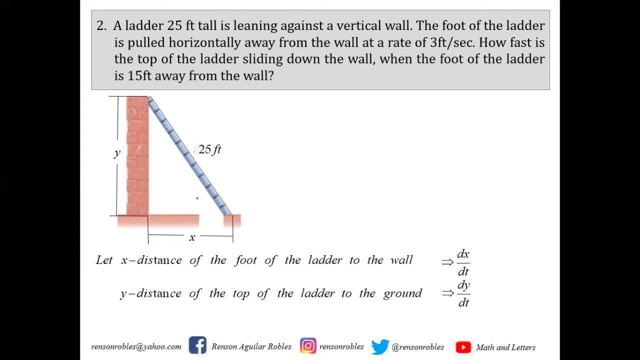 by some Pythagorean principle. here we shall notice that 25 squared equals x squared plus y squared and differentiating. so we have zero equals two x, dx, dt plus the differentiating y squared in terms of t, so that's two y dy dt and you can reduce this equation as: 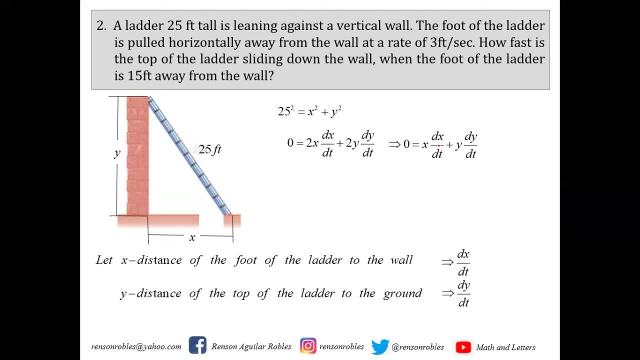 zero. you divide everything by two, so that's x dx dt plus y dy dt, and at a certain instant that dx dt is equal to three feet per second. okay, and x is equal to 15 feet. we shall now look for dy dt. dy dt again, is the rate of how fast the top of the ladder is sliding down or sliding up the wall. 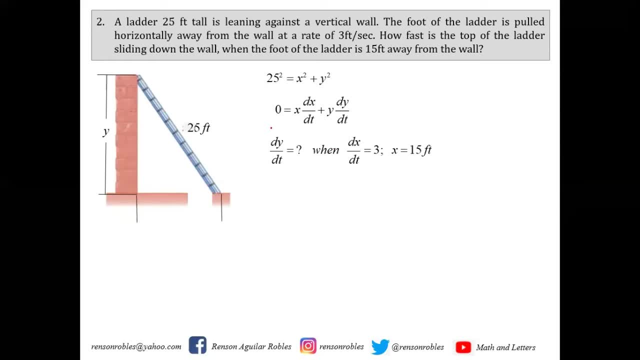 okay. so when you observe at the equation, our working equation is: zero equals x dx dt plus y dy dt, and we're looking for dy dt here. and dx dp is three and x is 15. so we shall now look for the value of pi at a certain instant that, uh, the foot of the ladder is 15 feet away from the wall. we 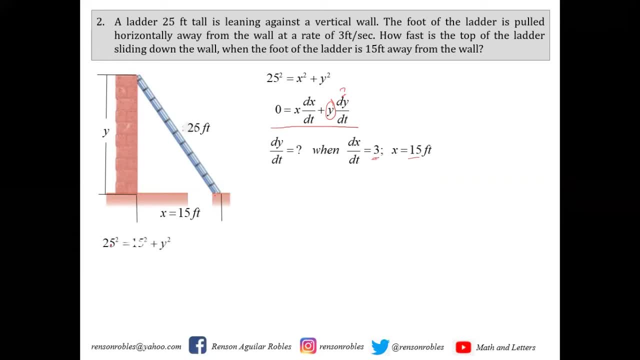 shall now compute for the value of y. so 25 squared equals 15 squared plus y squared, and it follows that y squared equals 25 squared minus 15 squared and y is equal to the square root of 625, that's, 25 squared minus 15 squared is 225, and 625 minus 225 is 400 and the 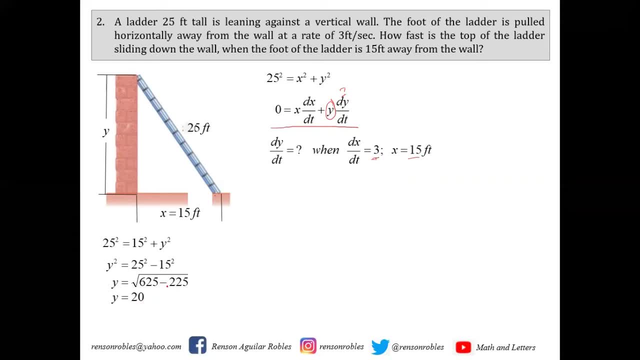 square root of 400 is 20.. so we have y equals 20 feet, and we shall now replace x by 15, the x dt by 3. y is 20 and d y dt is what we are looking for. so we shall now have 0 equals 15, that's x times 3, that. 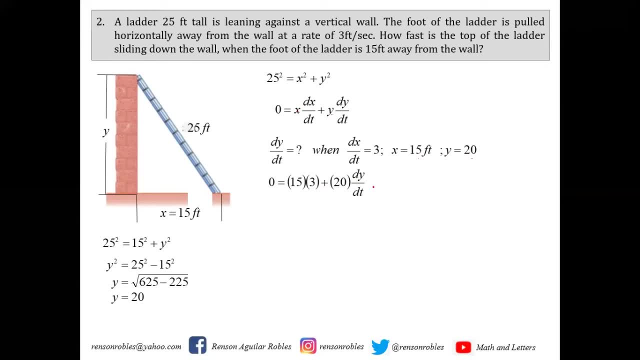 is your dx dt plus 20 dy dt and solving for dy dt, we shall have: dy dt equals 15 times 3 is 45. you throw it on the other side, so that's negative 45 over 1 and we shall have negative 9 over 4, 5th per second. 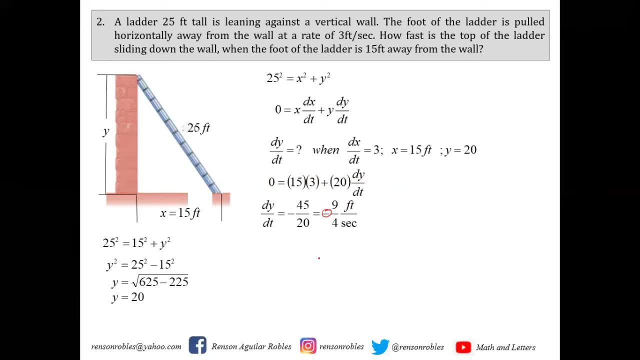 So this negative sign indicates that y decreases as the time t increases And, in conclusion, we can now say that the top of the ladder is sliding down the wall at the rate of 9 over 4 feet per second, when the bottom of the ladder is 15 feet away from the wall. 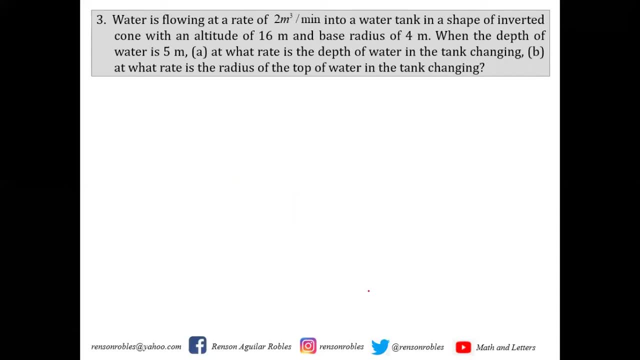 So problem number three: water is flowing at a rate of 2 cubic meter per minute into a water tank in the shape of an inverted cone with an altitude of 16 meter and base radius of 4 meter. When the depth of the water is 5 meter, we shall find for letter A, at what rate is the depth of the water in the tank changing, and letter B, at what rate is the radius of the top of the water in the tank changing. 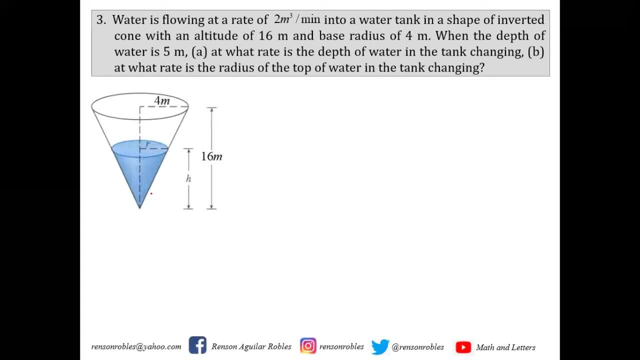 To illustrate here is the inverted conical tank with radius equal to 4 meter and altitude of 16 meter. So the water is being poured into the tank at a rate of 2 cubic meter per minute. So which means the VDT- the rate of how fast the water is flowing into the conical vessel- is 2 cubic meter per minute. 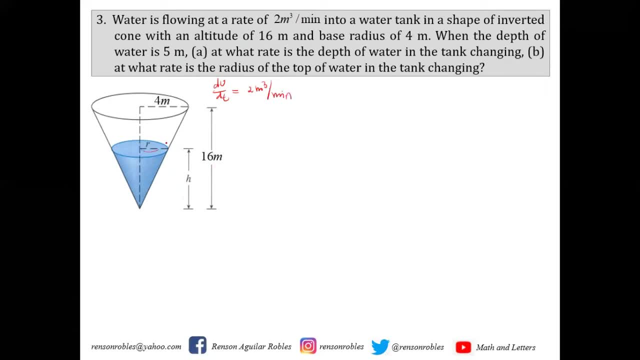 And we shall now let's. We shall let R to be the radius of the top of the water and H to be the altitude of the water. Okay, so we let H to be the depth of the water and R, and with its corresponding VHDT, to be the rate of change of how fast the water is, or the rate of change of the altitude of the water to the conical vessel. 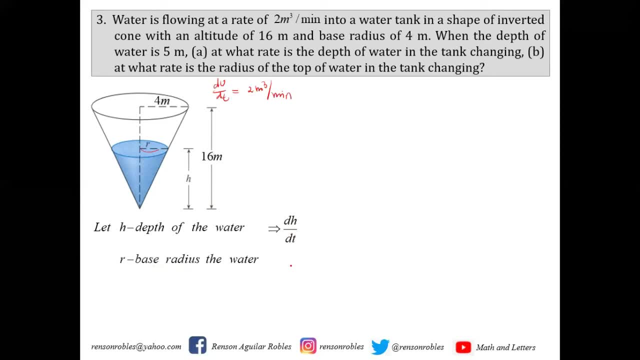 And R is the base radius of the water, which, With its corresponding rate of change, DRDT, And you will observe here that the rate of change of the rate of how fast the water is being poured into the conical vessel is 2 cubic meter per minute. 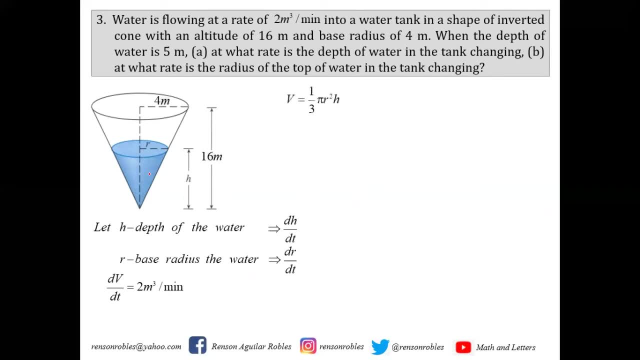 And we shall recall that the volume of cone is equal to one-third pi R squared H. And we shall now differentiate each variable here with respect to the time piece, So we have VDT equals differentiating R with respect to T, So we have one-third pi H, that's constant. and then the derivative of R squared is 2R DRDT. 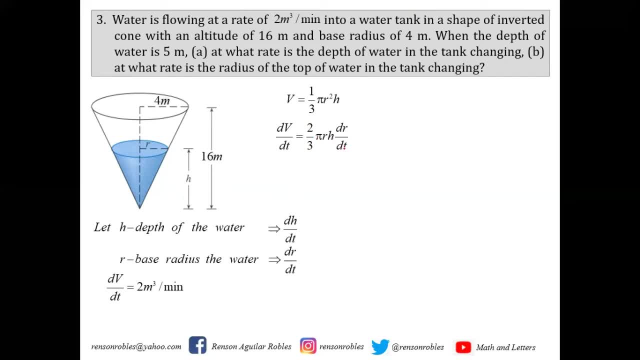 So that's why we have here two-third pi RH, DRDT Plus. we shall now do it again with respect. We shall now differentiate H with respect to the time T, So we have one-third pi R squared DH, And then at a certain instant that the volume that dVDT is equal to 2 and that the height of the water is equal to 5.. 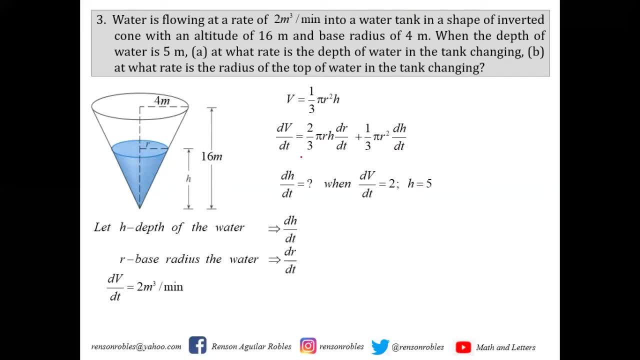 Okay, So we shall now use these quantities to substitute to our working equation. However, we only have dVDT, We have H, Okay, But we do not have DRDT And R On this specific situation. Alright, So what are we going to do now is to look for the value of R and DRDT so that we can now have our DHDT. 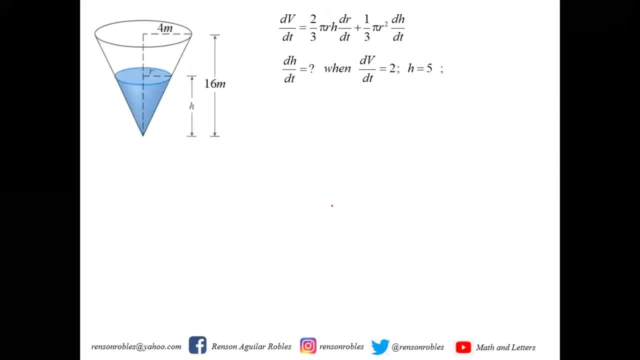 To do so by similar solid. we can now observe this relationship between H and R, that 16 over 4 is equal to H over R, And this follows that R is equal to one-fourth H. Okay, So we have. 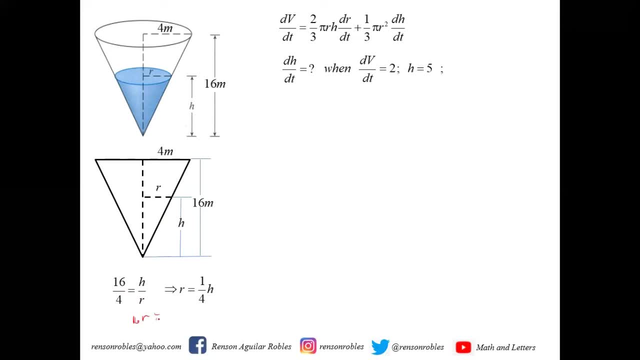 We have R times 16. So that 16R equals 4H. And then we divide everything by 16. So we have R equals 4 over 16H, And that will give us one-fourth H. 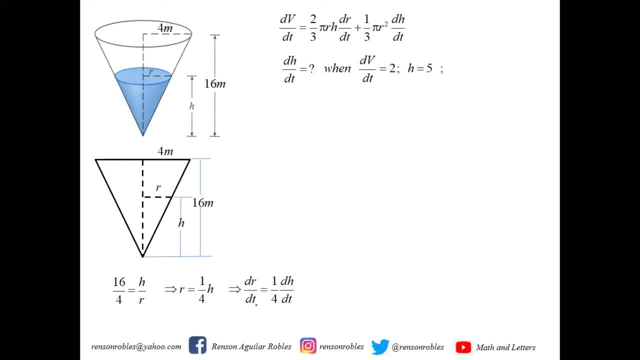 And then differentiating R with respect to T, we have DRDT. And then differentiating H with respect to T, we have one-fourth DHDT. So we shall now have DRDT equals one-fourth DHDT And we shall now look for the value of R whenever H is equal to 5.. 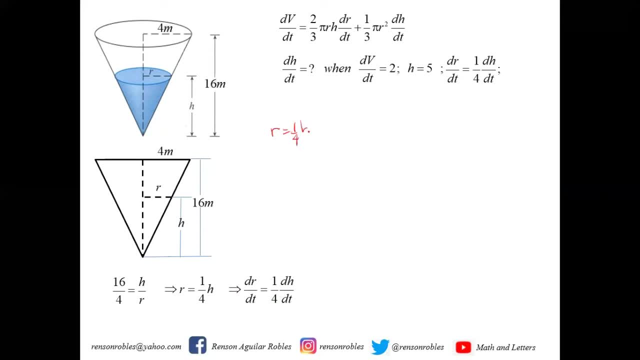 So we have R equals 1 over 4H, And when H is equal to 5 at a certain instant, so we have R equals one-fourth times 5.. So we have R equals 5 over 4 meters. 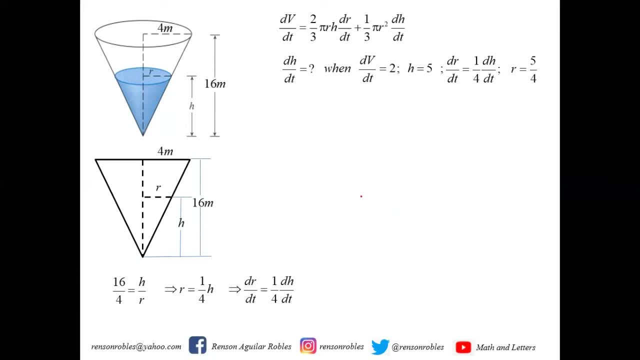 Okay, And then I think we are all set. So we have: DBDT equals 2.. Okay, And then 2.. One-third pi R is five-fourth times H, which is 5.. And then DRDT is one-fourth DHDT. 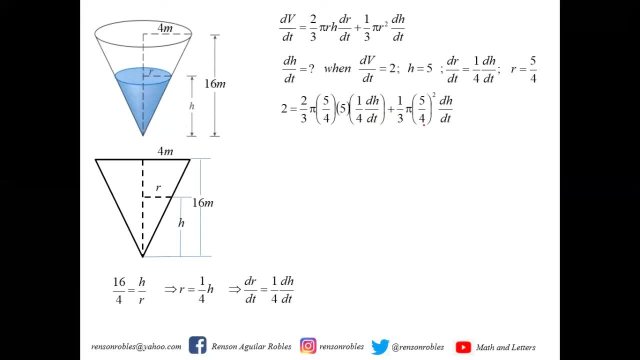 Plus one-third pi, Then R is 5 over 4 squared, Then DHDT, So we have 2, equals two-third times 5 over 4.. So again, I guess this is 5 times 5.. 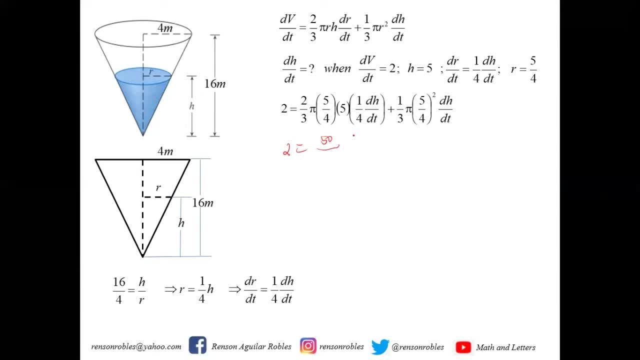 That's 25 times 2.. That's 50 over. Aha, This is 4 times 4. That's 16.. That's 48 pi DHDT. And then we have plus 5, squared, That's 25.. 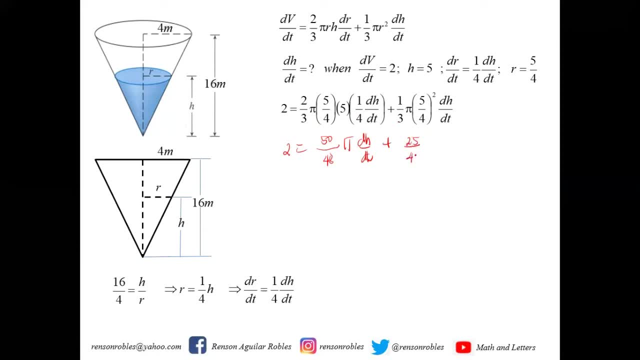 And then 4 squared, That's 16 times 3. We have 48 pi DHDT, And then we have 2 equals. combining these two, we have 75 pi over 48 DHDT, And then we can now say that DHDT. 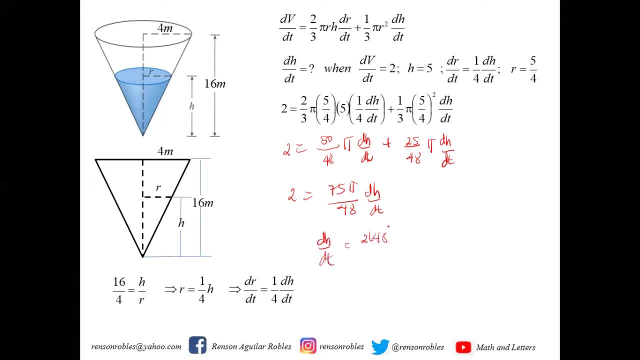 equals 2 times 48, all over 75 pi. Okay, And then we shall now have DHDT equals 32 over 25 pi, So 75.. We divide this by. We shall now divide this by 3. So this is 16.. 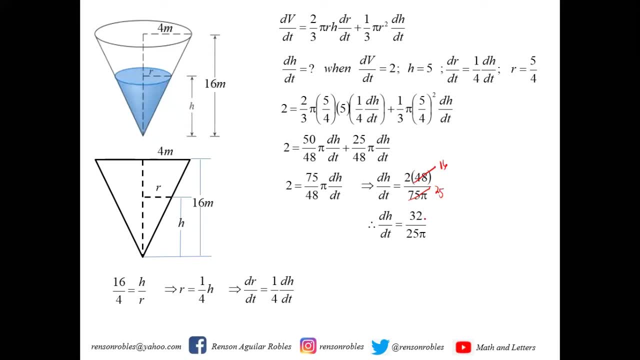 And this will become 25.. And 2 times 16,, that's 32 over 25 pi. Okay, So this is the rate of change of the altitude of the water with respect to the time. t For letter B, we are asked to find the rate of how fast the radius of the top of the water is changing. 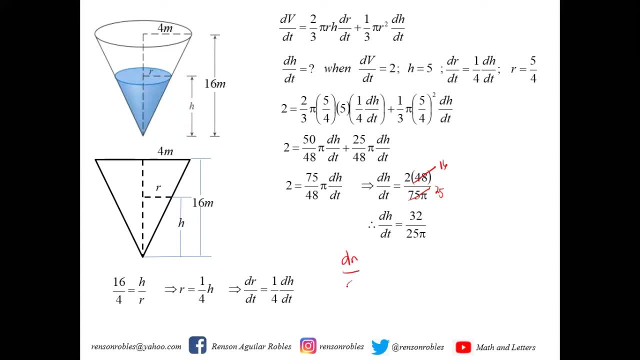 By using this principle, we now have DRDT equals 1 fourth times DHDT, wherein DHDT is 32 over 25 pi And 32 divided by 4. That is 8 over 25 pi. So this is our DHDT. 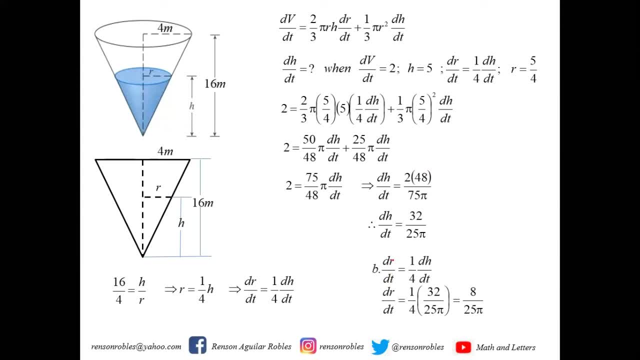 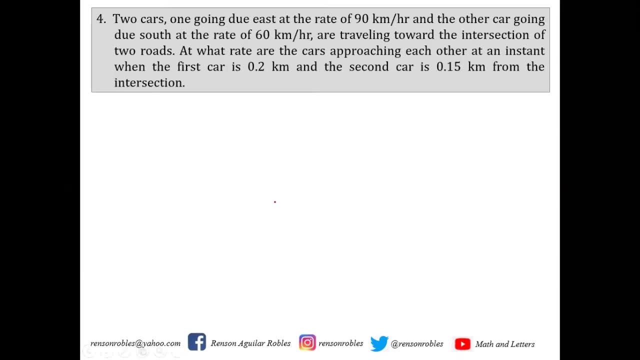 DRDT. sorry, That's the rate of the change in the radius of the water with respect to the time t, That's 8 over 25 pi. Problem number 4.. Two cars, one going due east at the rate of 90 km per hour and the other car going due south at the rate of 60 km per hour. 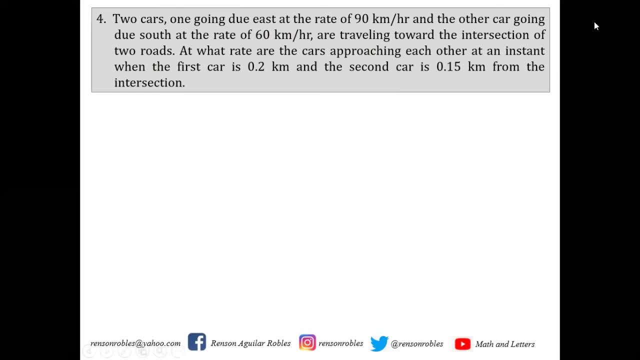 are traveling toward the intersection of two roads. At what rate are the cars approaching each other at an instant when the first car is 0.2 km and the second car is 0.15 km from the intersection? To illustrate, let us assume that this is the intersection of the two roads. 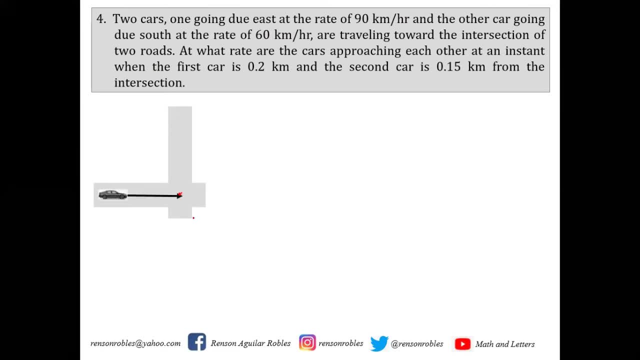 And the first car is traveling due east at the rate of 90 km per hour And the second car is traveling due south And the second car is traveling due south at the rate of 60 km per hour. So the two cars are traveling toward the intersection. 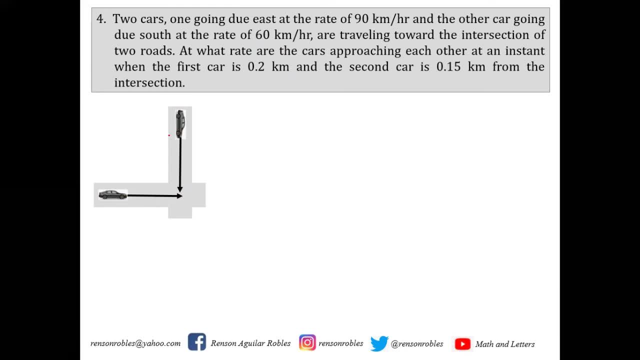 So there will come to a point that the distance between the two cars will be somewhere here at this point, And the second car will be somewhere here at this point, And we shall now let x to be the distance of the first car to the intersection. 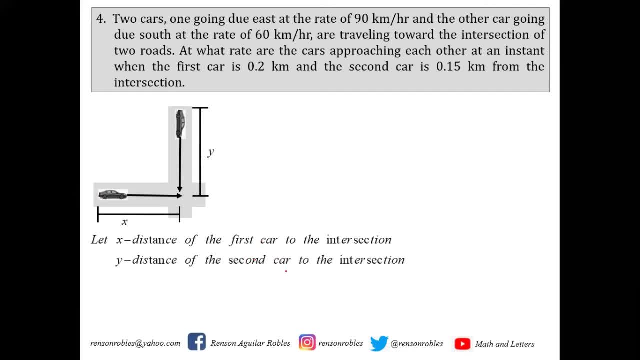 And y to be the distance of the second car to the intersection, And we shall now let z to be the distance of the two cars as they approach the intersection, And this has a corresponding rate of change. We see that dx, dt, that's the rate of how fast the first car is approaching the intersection, that's 90 km per hour. 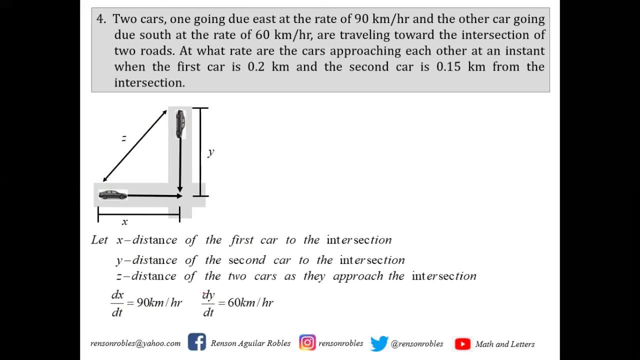 And then the rate of how fast the second car is approaching the intersection is 60 km per hour, And we shall now let dz dt Okay To be the rate of how fast the two cars are approaching with each other. So by Pythagorean principle, we can now see that z squared equals x squared plus y squared. 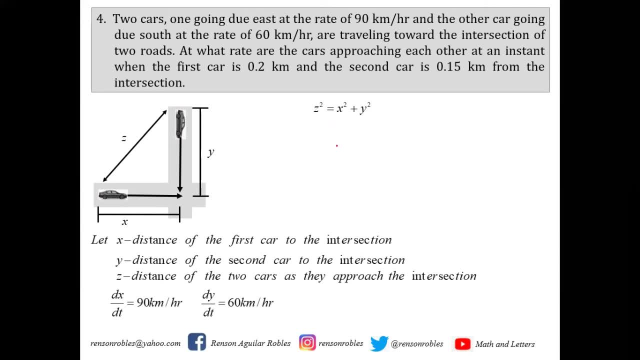 And then differentiating all this variable with respect to the time t, we shall now have 2z dz dt plus 2x dx dt plus 2y dy dt, And you can observe that each term contains two. So we can now. 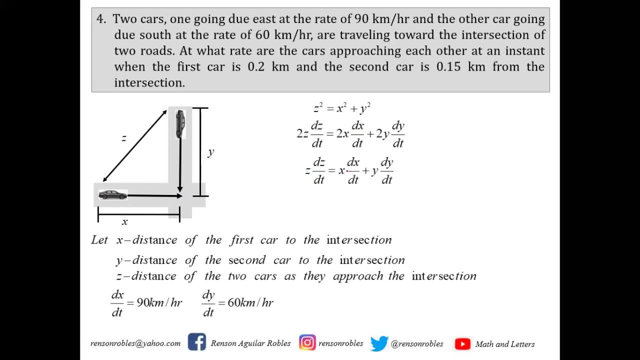 So we can now reduce this of the form z, dz, dt equals x, dx, dt plus y, dy, dt And, at a certain instant, that the first car is 0.2 km away from the intersection and that the second car is 0.15 km away from the intersection. 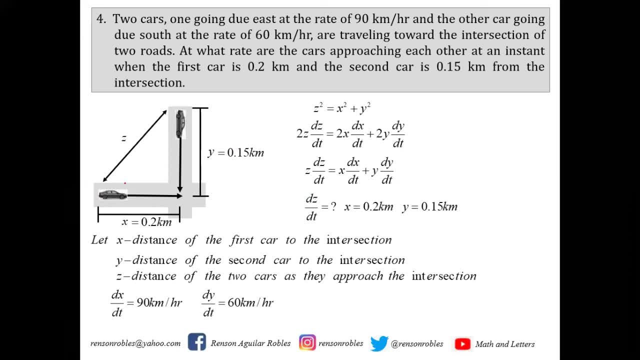 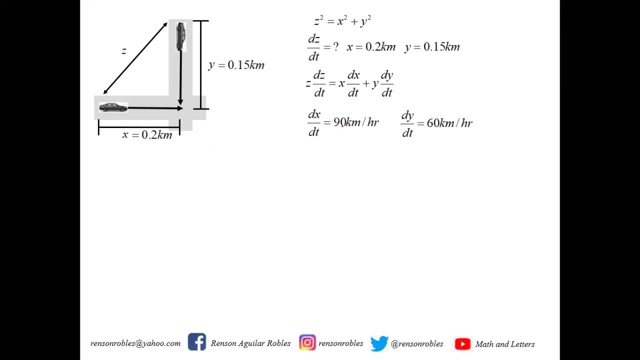 we shall now be looking for the rate of how fast these two cars are approaching each other. Okay, So, at a certain instant. So at a certain instant, we shall now look for the value of z. As you can notice, in our working equation we have z, dz, dt equals x, dx, dt plus y, dy, dt. 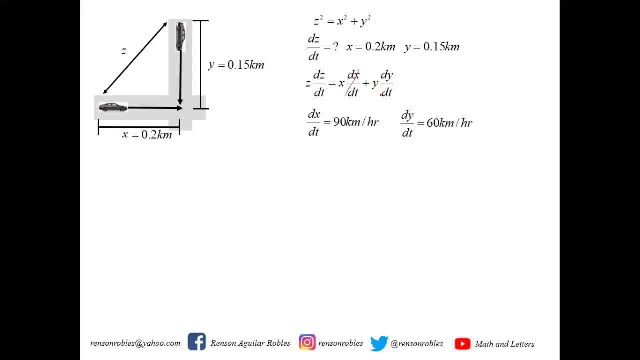 So we already have our dx dt, We already have our dy dt, We now have our x and y And we shall now look for dz dt. but we do not have this value of z. Okay, By Pythagorean principle, we shall now have z squared equals x squared. 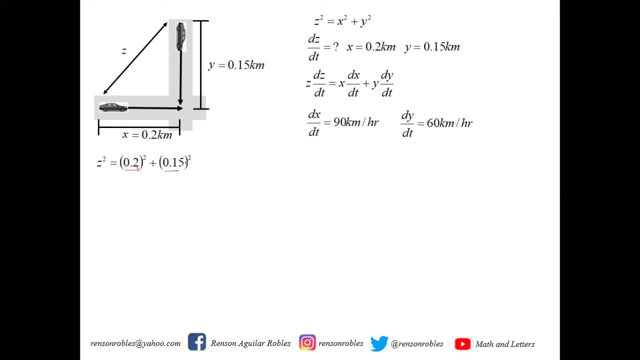 That's 0.2 squared Plus y squared, That is 0.15 squared, And simplifying this, we shall have: z equals the square root of 0.2 squared plus 0.15 squared, which is equal to 0.25 km. 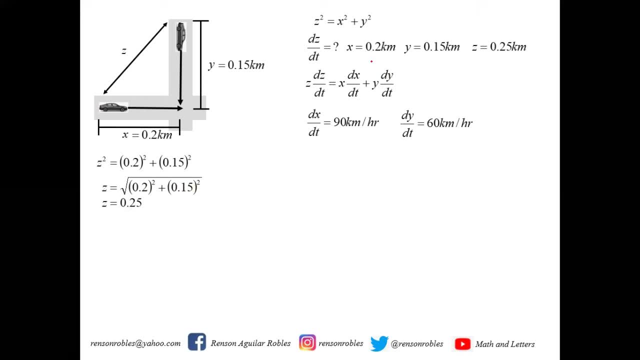 So, at a certain instant that the first car is 0.2 km away from the intersection and that the second car is 0.15 km away from the intersection, then the two cars are 0.25 km away. And then, substituting these quantities to our working equation, we shall have z, that's 0.25 times dz. dt equals 0.2 times negative 90. 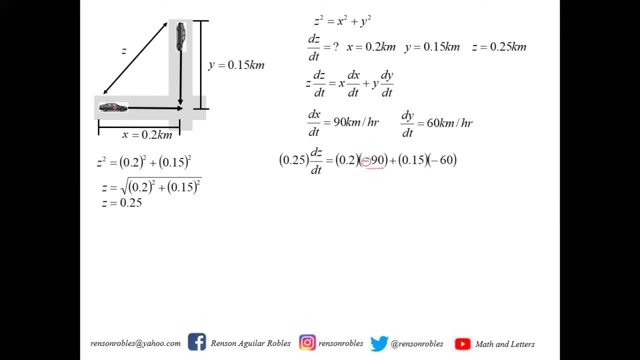 I affixed the minus sign here because, as you can observe, as the first car approaches the intersection, their distance decreases And therefore the rate of how fast the car approaches The intersection will be negative. Same with dy dt, which is equal to 60 km per hour. 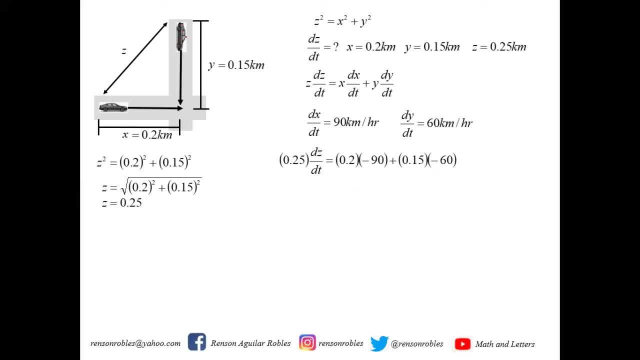 We shall affix the minus sign, since this car is going due south and its distance gets smaller and smaller as it approaches the intersection. So we shall have 0.25 dz. dt equals 0.2 times negative 90 plus 0.15.. 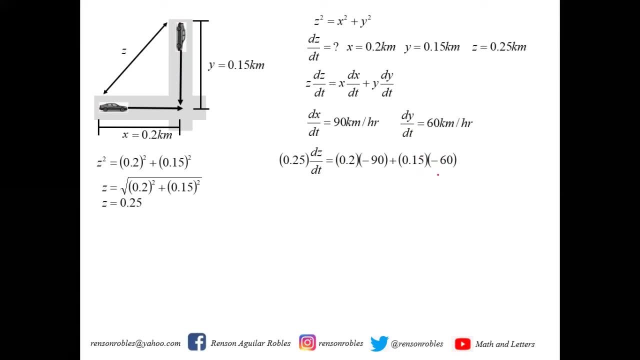 That is our y Times, dy dt, which will become negative 60. And, as you can notice, as these two cars approach the intersection, their distance will decrease. At a certain point that the second car is located somewhere here, that the first car is located somewhere here, then their distance gets smaller. 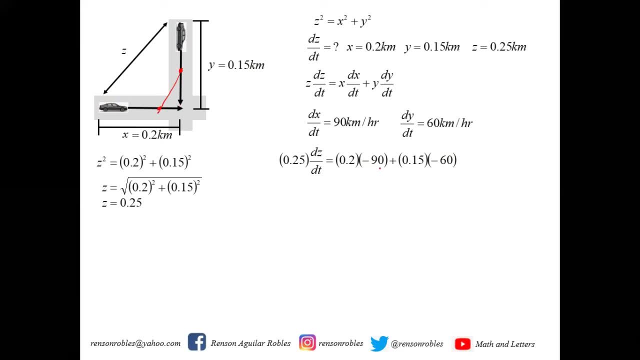 That's why we have negative here, here and negative 60.. And then, looking for dz dt, we shall have 0.2 times negative 90 plus 0.15 times negative 60, divided by 0.25.. 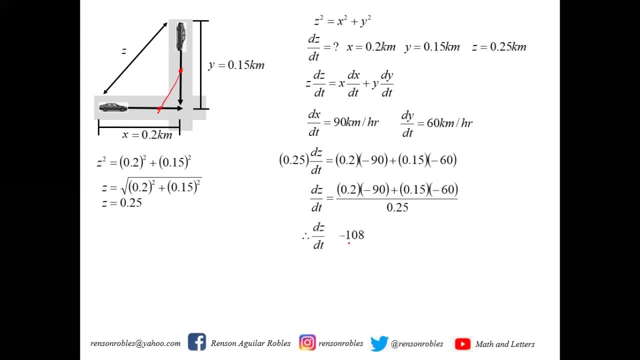 And executing this on your calculator, we shall have dz. dt equals negative 108.. And this negative indicates that the distance between the two cars gets smaller and smaller as they approach the intersection. So, in conclusion, the two cars are approaching each other toward the intersection. 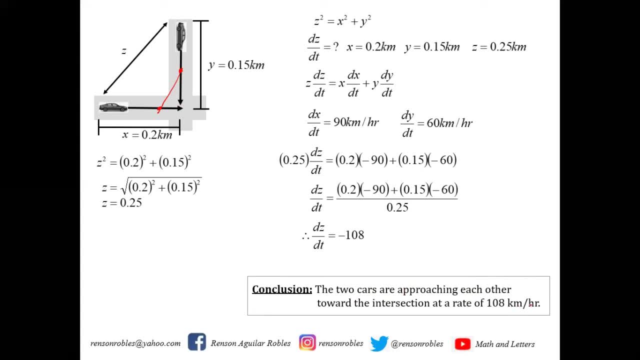 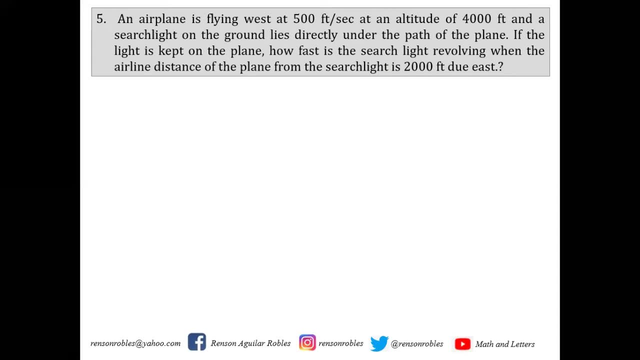 At a rate of 108 km per hour. And last problem: An airplane is flying west at 500 feet per second at an altitude of 4,000 feet and a search light on the ground lies directly under the path of the plane. If the light is kept on the plane, how fast is the search light revolving when the airline distance of the plane from the search light is 2,000 feet due east? 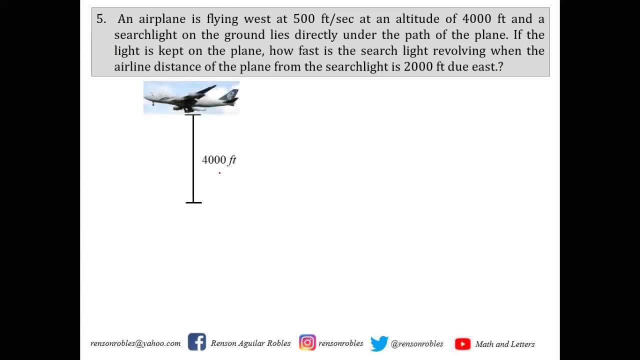 Okay to illustrate. there is a plane which is 4,000.. 2,000 feet from the ground and under the path of the plane, there is a search light which follows the airplane, And we shall let the time t to be the time that has elapsed since the search light spotted the plane. 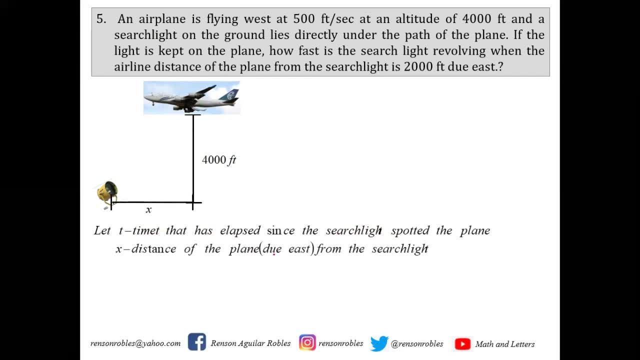 And x to be the distance of the plane due east from the search light, And y- Oh Sorry- And theta. We have an angle, theta To be the angle of elevation to the plane of the plane at the search light. okay, and as you can notice here, we can now have our dx dt, which 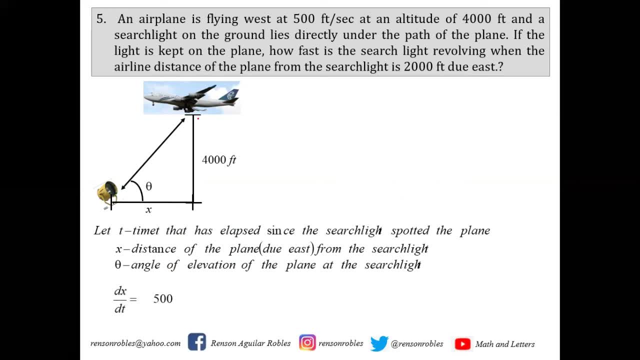 is equal to 500 feet per second. and do not forget that the uh airplane is flying west. that means to the left. okay, so we shall now affix the minus sign. okay, and d theta, dt is what we are looking for. whenever x is 2000 feet, whenever the the distance of the airplane to the search light is 200 feet. 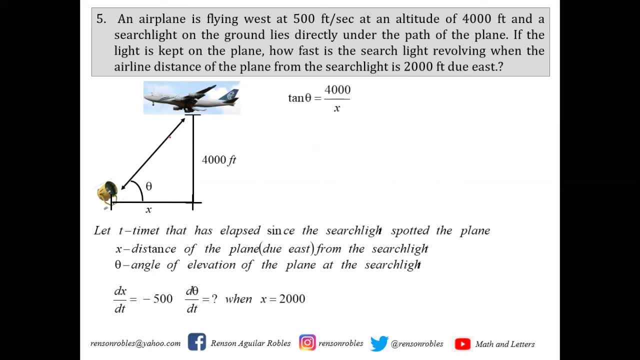 so again by the Sukhothoi principle, since we can now observe a right triangle here. we now have: tangent theta equals 4000 over x and then, differentiating this, we have second squared theta: d, theta d, theta dt equals negative 4000 over x. squared dx dt, that's the derivative of 4000 over x in terms of t. okay, and then therefore: 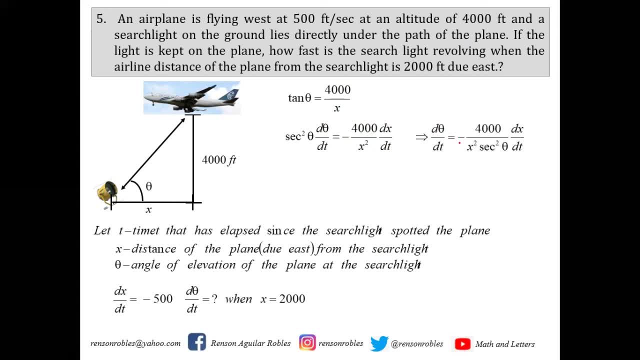 we can now say that d theta dt equals negative 4000 over x squared secant squared. theta dx dt. d theta dt again is the rate of how fast the search light is revolving when the airline distance of the plane from the search light is 2000 feet. due is Okay to do this. we shall now have. 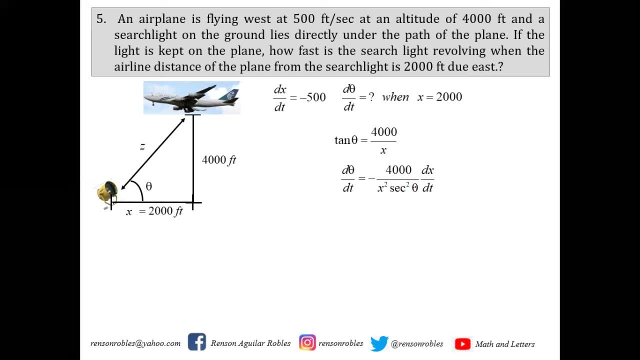 to look for the value of secant squared theta at an instant where in x is 2000 feet and again by using this principle, tangent theta equals 4000 over x. we can now see that when you replace x by 2000, we have tangent theta equals 4000 over 2000.. 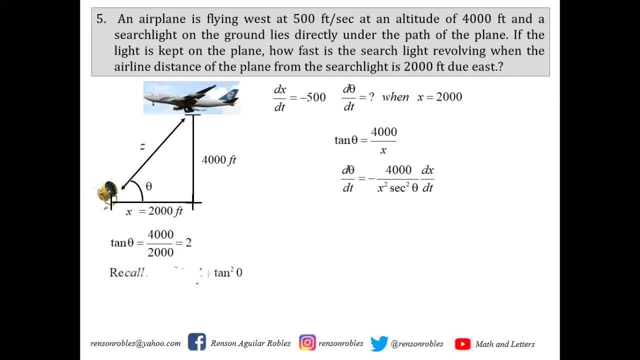 thousand, which is equal to two. and then you recall that secant squared theta equals one plus tangent squared theta, and we shall now have secant squared theta equals one plus you replace tangent theta by two, so we have two square. that's your tangent squared theta, and it follows that secant squared 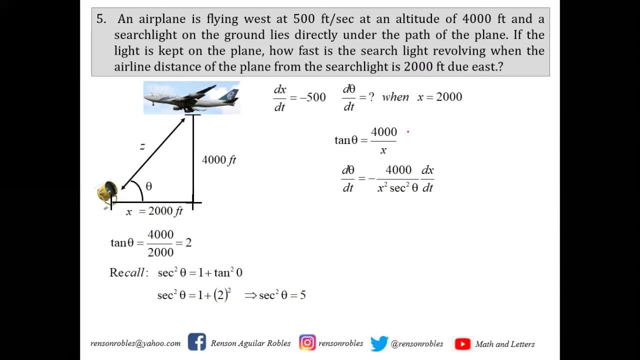 theta equals five. so we shall now look for d theta dt whenever x is two thousand, whenever secant squared theta is five and that dx dt is negative five hundred. so d theta dt equals negative four thousand, all over two thousand squared times five, times negative five hundred. and executing this on